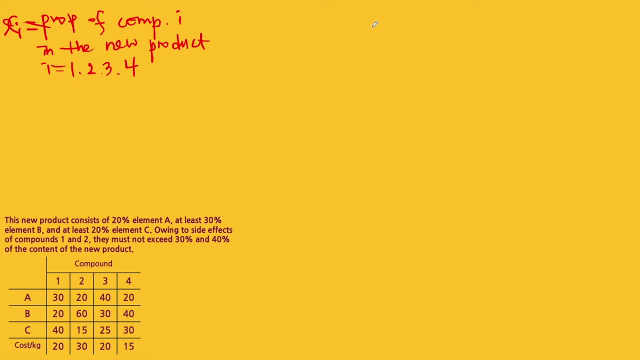 We say in the previous slide, the objective function would be the total cost of the compounds. So the total cost of compounds comes from the last line of this table, So 20x1,, 30x2,, 20x3,, 15x4.. 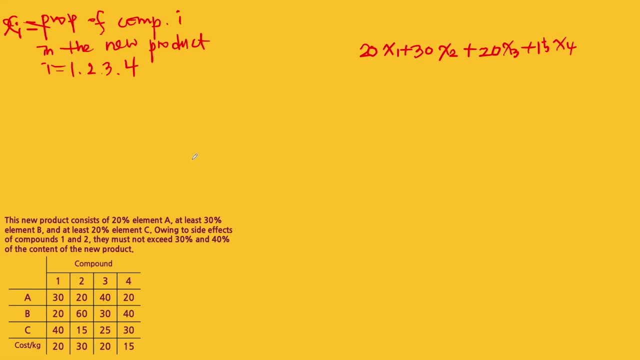 So 20x1 incurred from compound 1 and 30x2 is the cost incurred from compound 2 and etc. And then we are going to minimize this And then we want to. We want to write down the constraint here. Here the first constraint is: the new product consists of 20% of element A, exactly 20%. 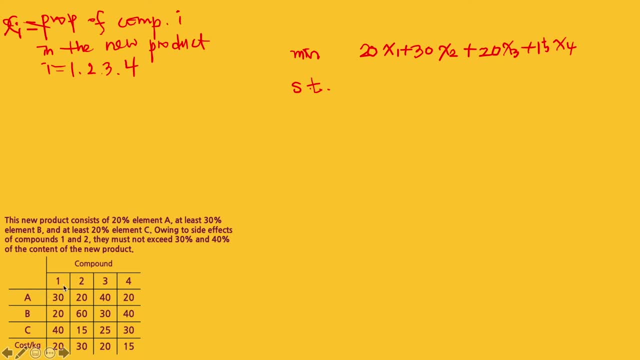 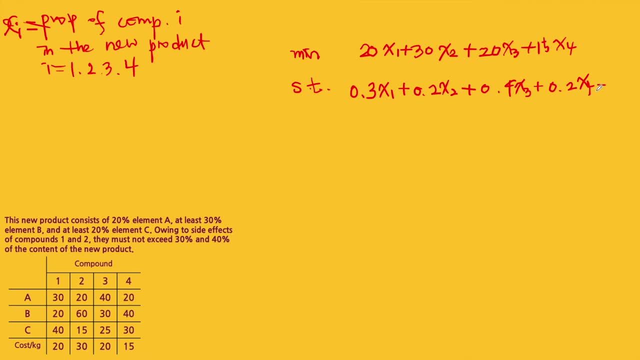 0.2x4., 0.2x4., 0.2x4. 0.2x4., 0.2x4., 0.2x4. 0.2x4.. That is 0.2.. 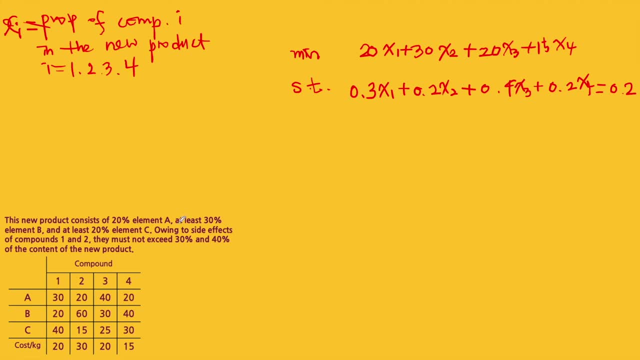 And the next one would be the proportion of element B That is at least 30%, So 0.3 and greater than equal to, And then same as the element A. We can write, write down as 0.2x1, 0.6x2, 0.3x3, and the last one would be 0.4x4 and the 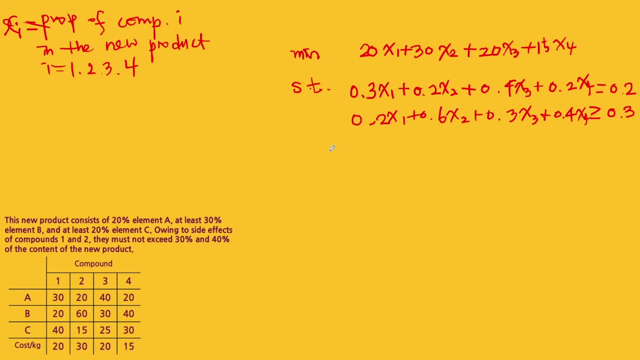 next one is the proportion of element C. so you read this part right. the third row of the table: 0.4x1, 0.15x2, 0.25x3 and the last one is 0.3x4, that is: 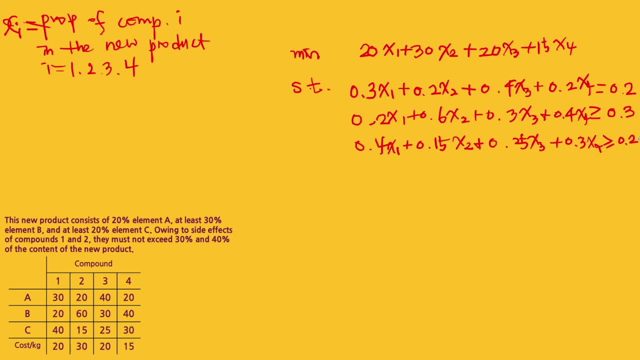 greater than equal to 0.2, and then the proportion of the compounds 1 and 2 cannot exceed 30% and 40% of the new product. so we are going to write down here: x1 cannot exceed 0.3 and x2 cannot exceed 0.4. and then we are also: 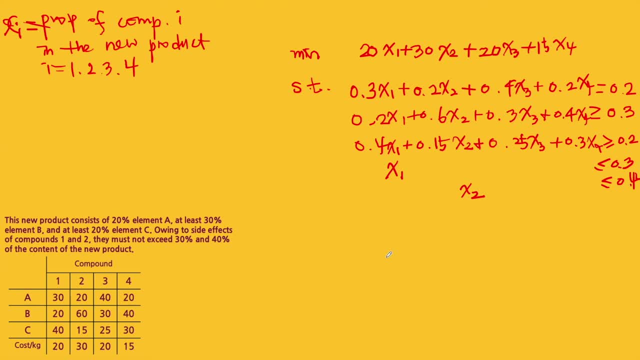 supposed to write down the domain of decision variables. here we cannot find explicit information about the domain of the variable, but we can see that these values- x1, x2, x3, x4- are non-negative. so this is a complete form of the mathematical formulation. it might be. 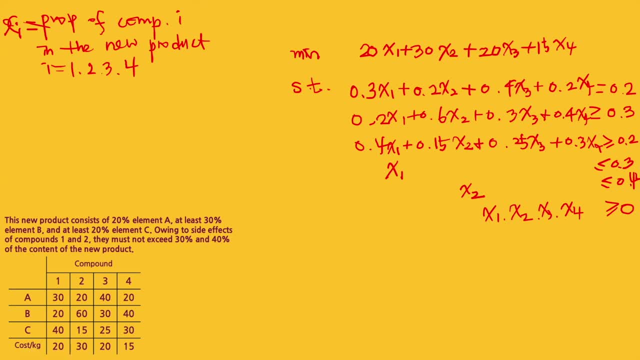 confusing at the first time, but you will know it for yourself. thank you, see you next time. if you keep practicing, you can write down any mathematical model formulation easily. and if you want me to solve some problems or write down the mathematical model formulation, please leave them in the comments. thank you for.